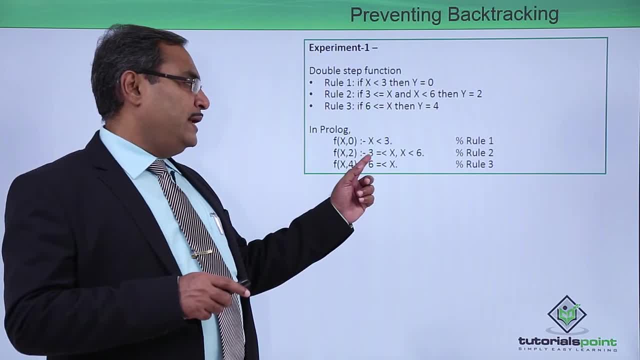 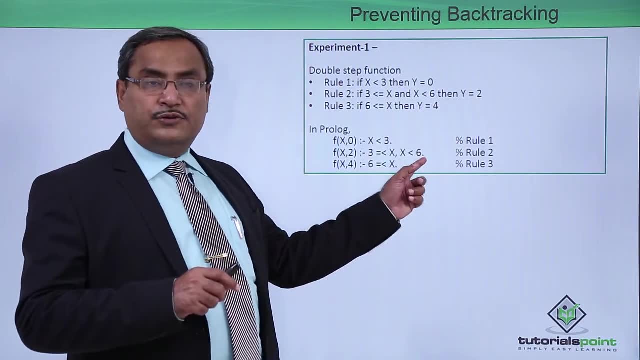 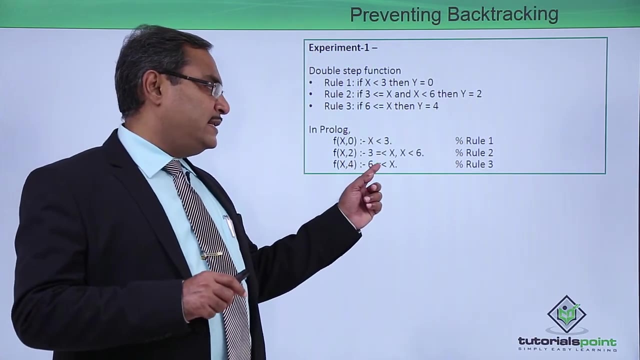 than 2, if x produce output 2,. if 3 is less than equal to x and comma means and x is less than 6, full stop. x will produce output 4, if x 4, if 6 is less than equal to x. So 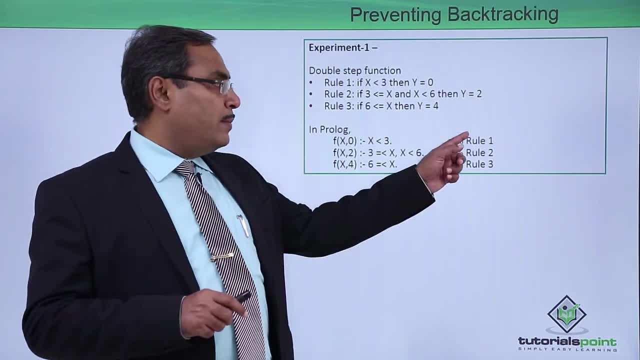 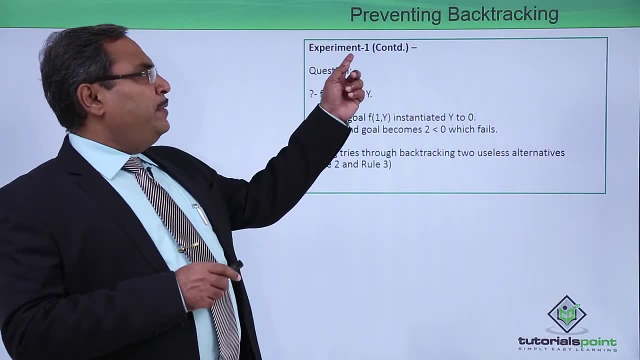 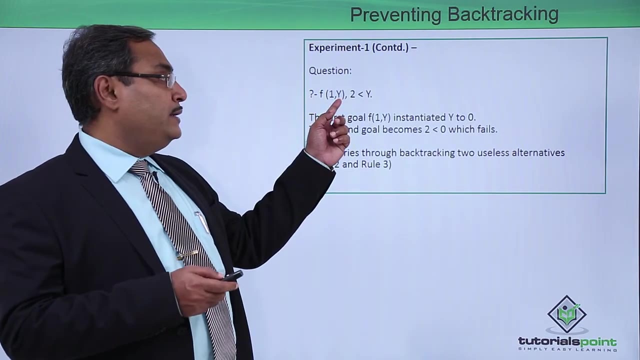 we have written the same in our prologue syntax. That is our rule number 1, 2 and 3.. Percentage denotes that they are the comment lines. Question number 1 continued. Question f 1: y. So I am asking the value of y If y is. 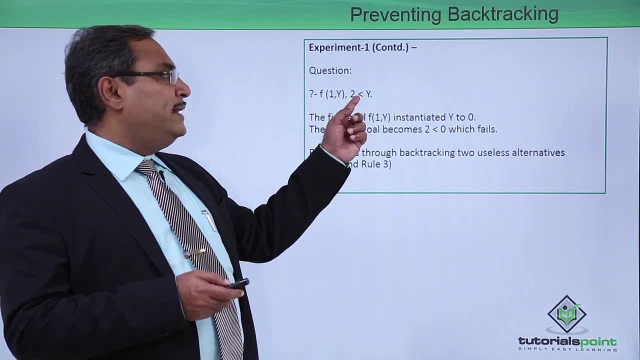 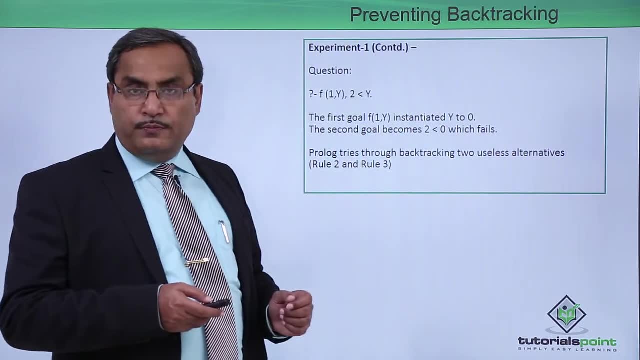 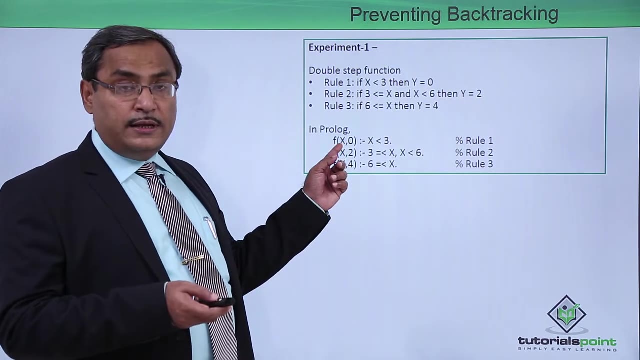 greater than 2 and 2 is less than y. the first goal, f 1 y, instantiated y to 0 because in the first goal we had that x is less than 3, then obviously we can have the value of x will become 0.. 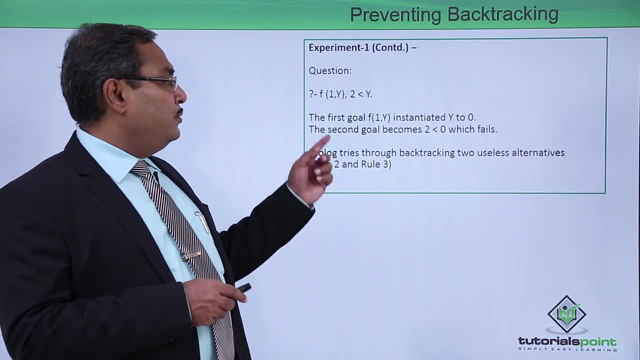 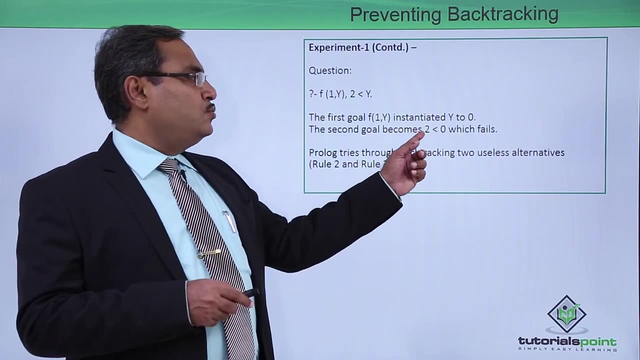 So that is, the output will be 0, rather, in this case. So now the first goal, f 1 y, instantiated y to 0.. The second goal becomes 2 less than 0, which fails. Prologue tries through backtracking. 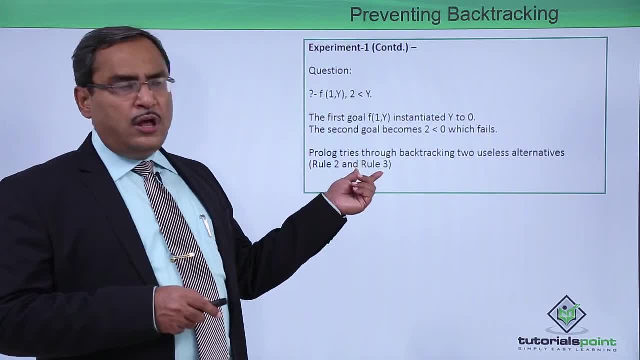 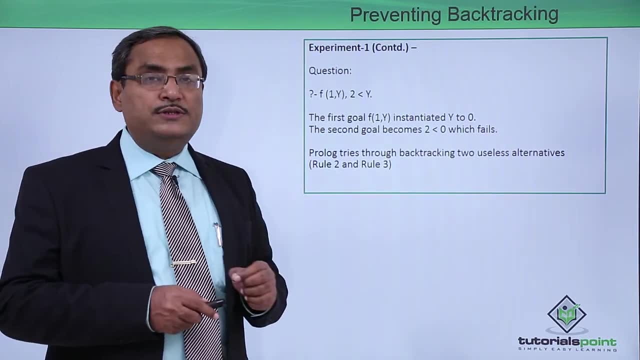 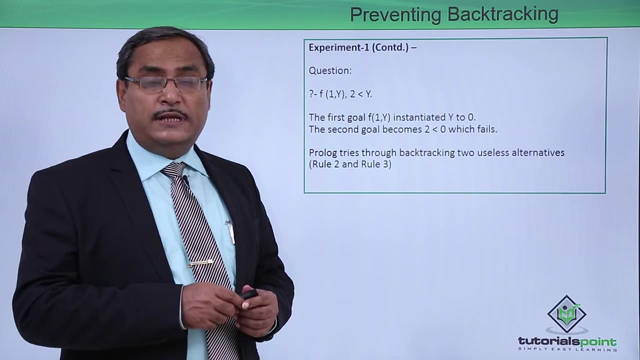 two useless alternatives, rule number 2 and 3, where rule number 1 has got already been satisfied and the respective y has got instantiated with the value 0. So that is why here this backtracking is unnecessary And time consuming, increasing the complexity of the respective prologue program execution. 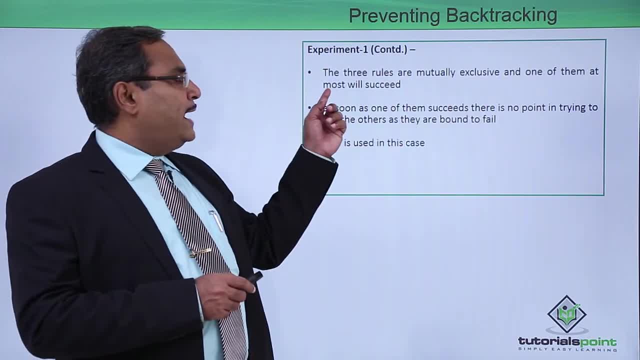 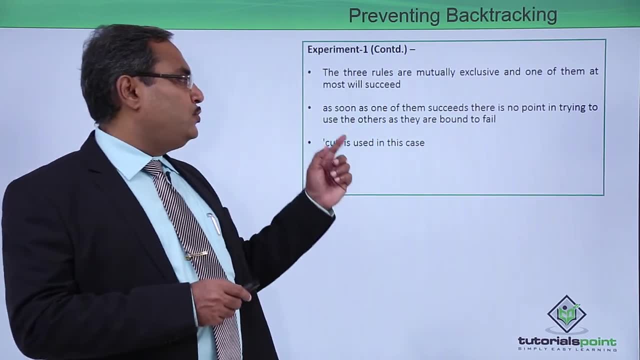 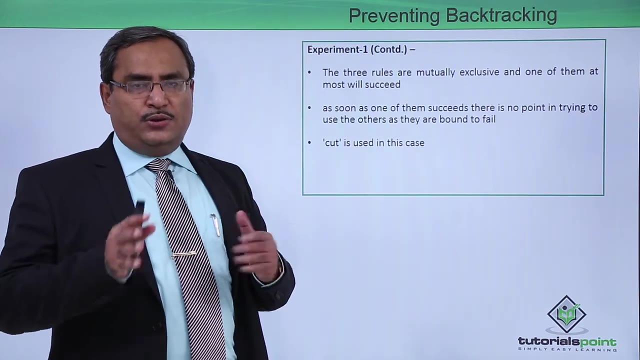 The three rules are mutually exclusive and one of them at a time. most will succeed. As soon as one of them succeeds, there is no point in trying to use the others, as they are bound to fail because all the rules are mutually exclusive. So if one of them is, 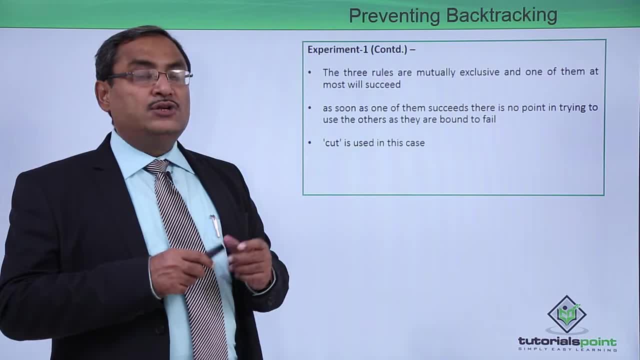 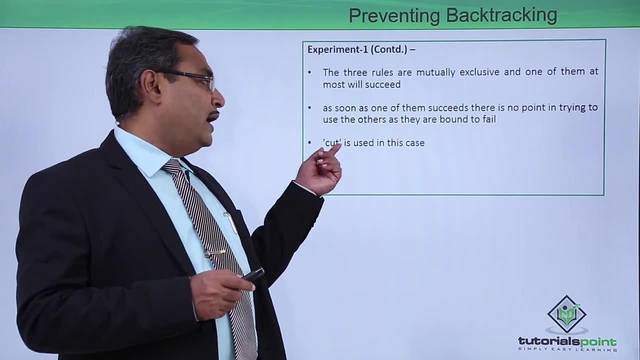 getting satisfied, then other rules cannot get satisfied. So that is why if one of the rules is getting satisfied, then I should not try with the other alternatives available. Cut is used in this case. So now we are going to introduce cut, which will prohibit. 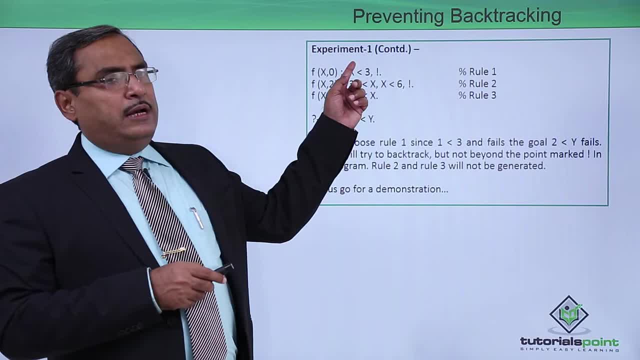 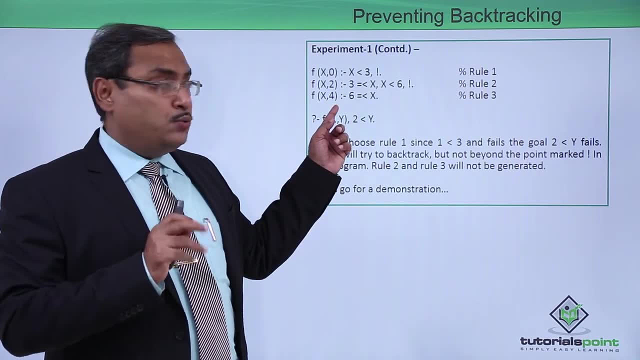 our backtracking. Let us continue with this experiment number 1.. Here we have written the same clauses, the same rules we have written, but we have added something new. After this: x less than 3 comma means AND one symbol. we have input here. 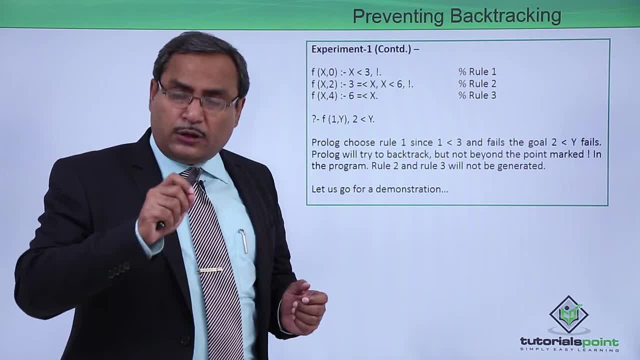 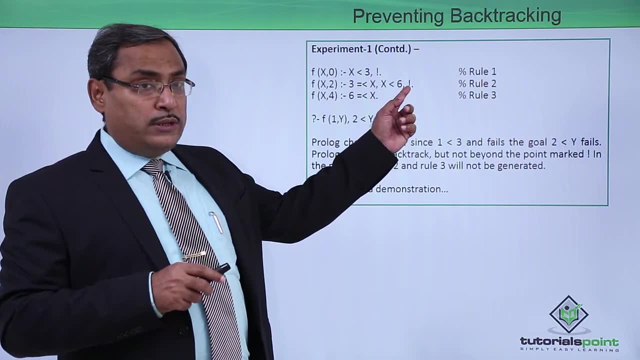 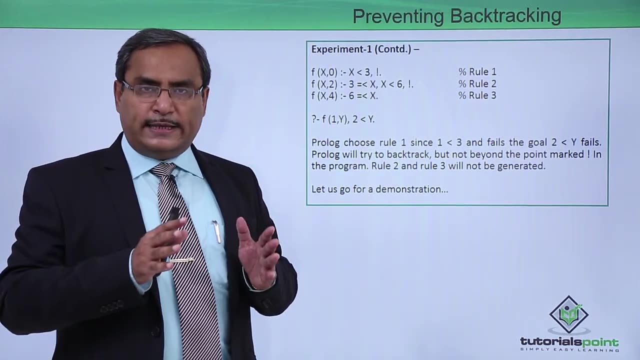 We have included here, known as the cut. So cut will be represented by this symbol: exclamation. So here also, AND cut. So we know that in this case only one rule will get executed, because rules are mutually exclusive. So one rule will get executed, all the rules. 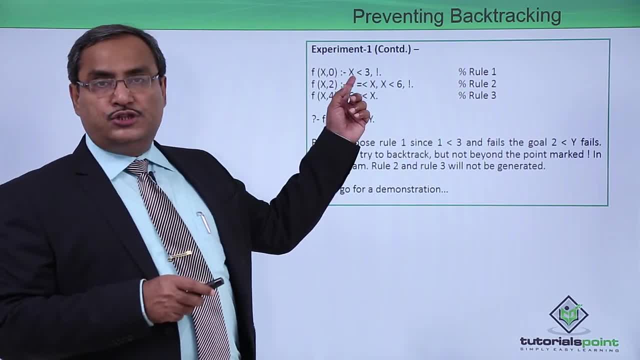 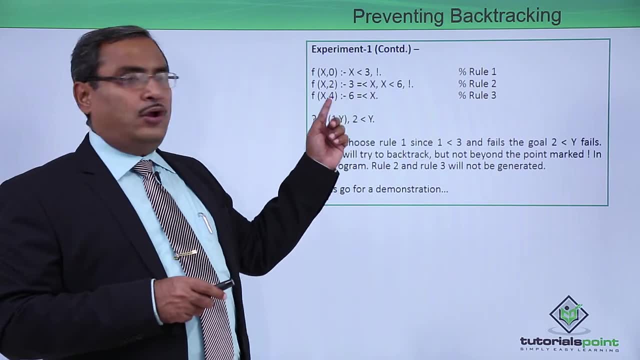 cannot get executed at the same time. So whenever this condition is true, then cut will get executed and it will prohibit to do the backtracking and checking with other clauses. that's why this cut will give us the correct answer which i was also getting in the previous. 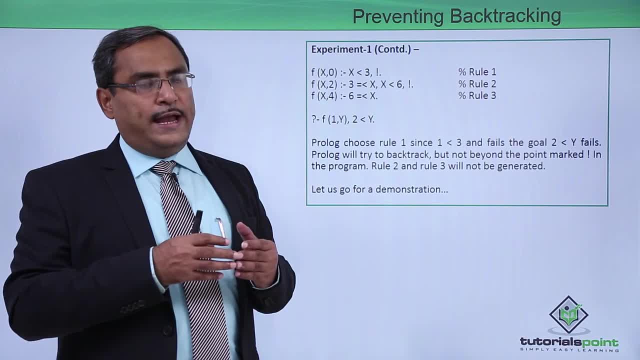 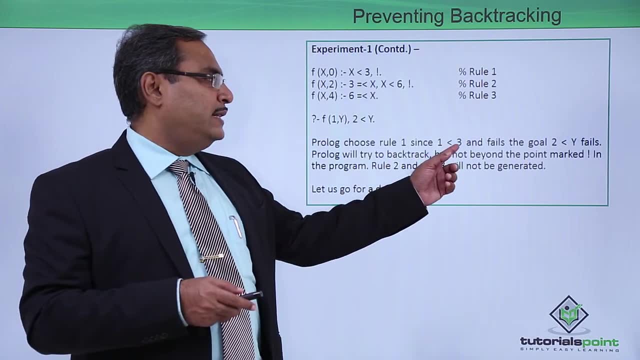 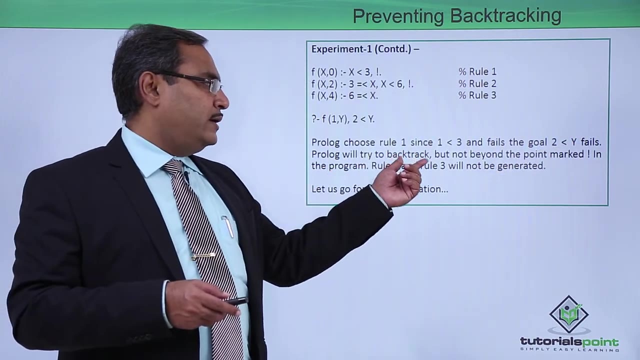 version, but in a faster way because it will not go for any kind of unnecessary checking with the other clauses. prologue: choose rule one since one less than three and fails the goal. two less than y fails. prologue will try to backtrack, but not beyond the point marked by this exclamation. 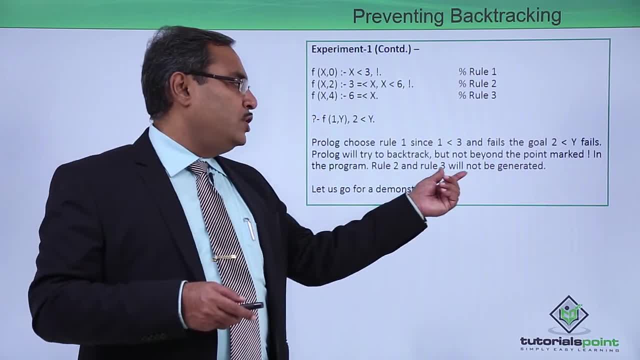 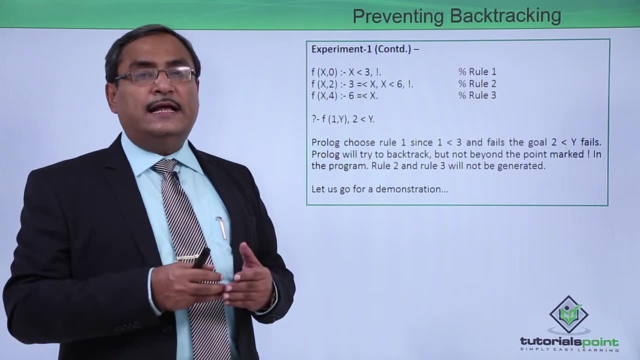 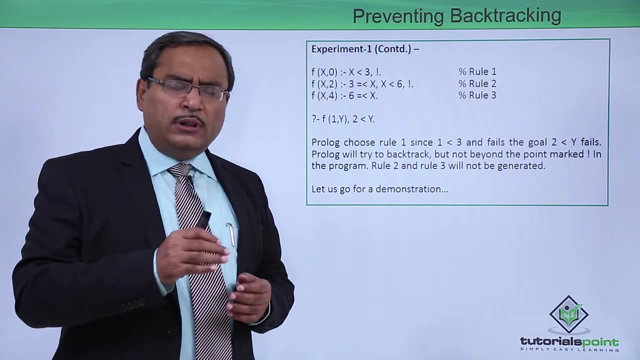 in the program, rule two and rule three will not be generated and executed how. that will bring us faster answer, getting the answer in a faster way in the minimum time, and that will bring optimality in my code. so for all these issues, let us go for one practical demonstration where we shall show. 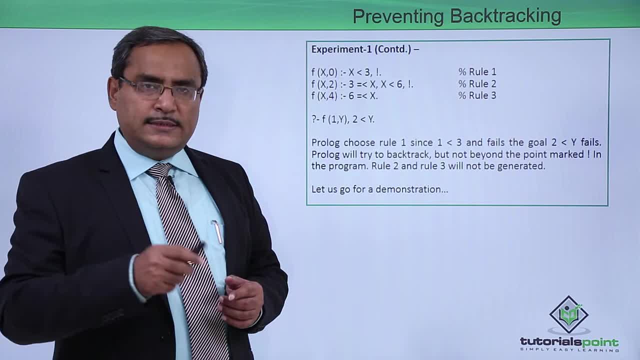 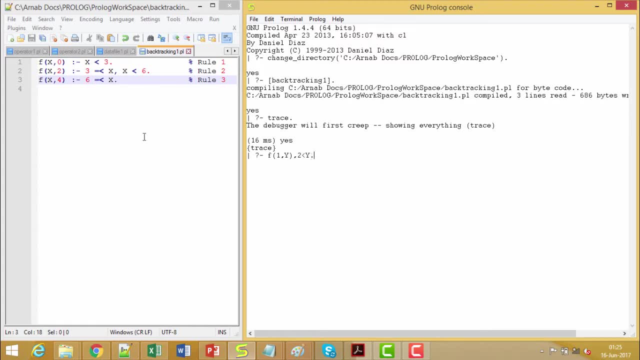 you all these things into more details. here is the demonstration for you. so here is the practical demonstration of this prologue program. so this is our code. the program has been compiled and loaded into the memory. the trace is on and here is the query or goal for us. so f one comma y, comma two less than y so here. 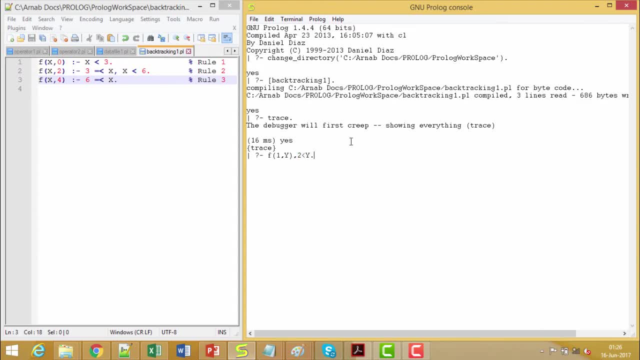 comma denotes the end operation. okay now, if i execute this query, so at first it is calling this one comma, this y, so it will be called at first. so then one less than three. so it has to be checked. so one less than three will be okay, so exit with one. 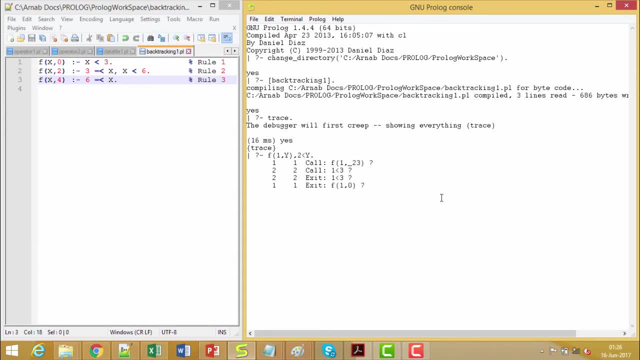 less than three, as true, so now. so exit with f one zero. so here we are getting this one. so here we are getting this one. and as this right hand side is true, so it is exiting with: y is equal to zero here, so y is equal to zero accordingly. so now it will check the rest part of my query, that is. 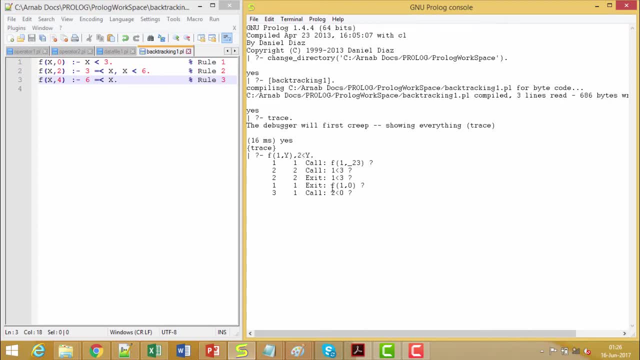 two less than y. so here y is equal to zero. so two less than zero is being checked. that will be false. so fail has occurred. so now we are having this redo. that is f one zero. so now it is calling three less than equal to one. so here you see, it is a redundant check. it is not at all required. so in 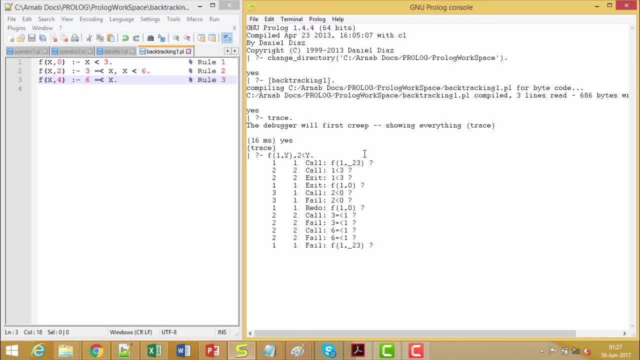 this way, the rest part will be executed. i'm showing you the output accordingly. so it is failing ultimately and giving the answer no or false. okay, now let me put one cut symbol here, so saving this, going for no trace coming out from the debugger mode. so now i'm going for the compilation and reloading of the code. so it is okay for me. it is uh, back. 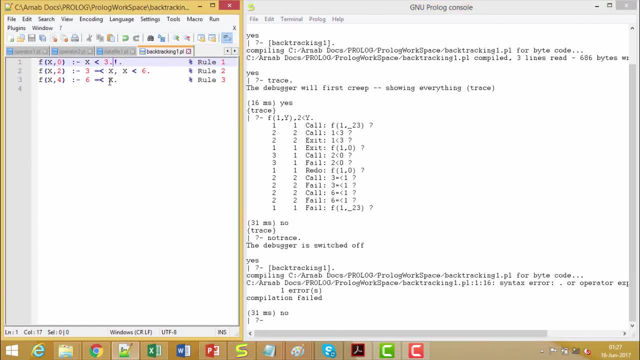 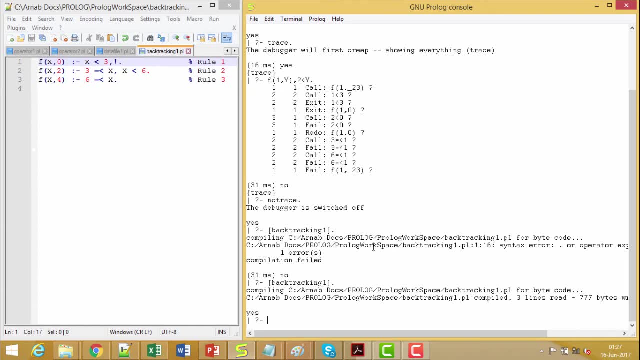 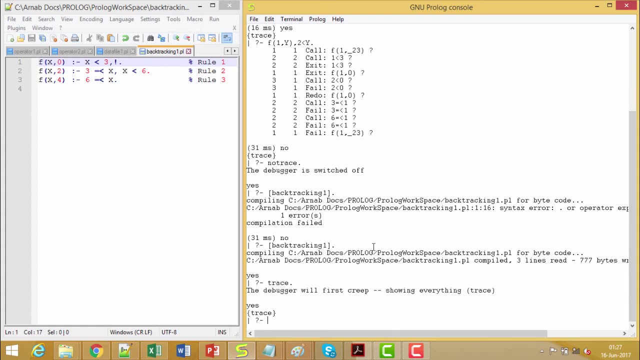 tracking. one has got this. okay. that is one error, is there? so putting this one as comma? that is quite obvious. this is an error. so now let me go for this. respect are keeping. now the code is compiled, okay, and it is now in the memory so I can make. 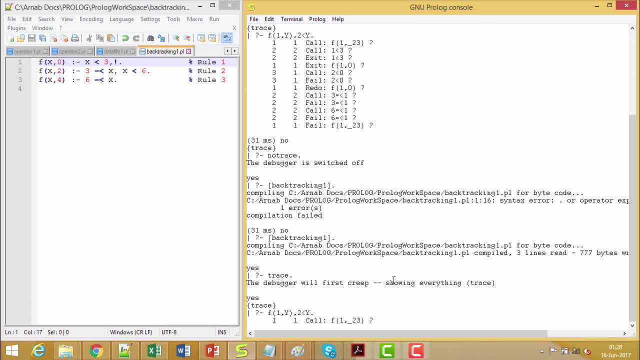 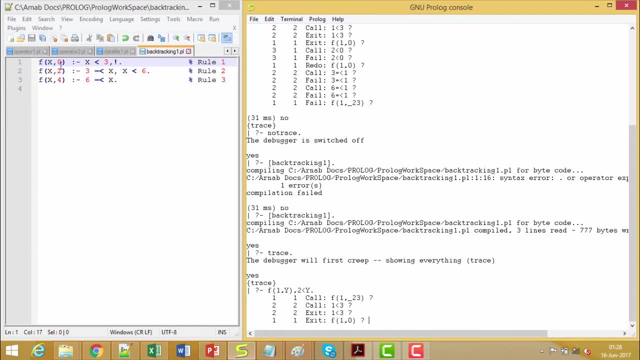 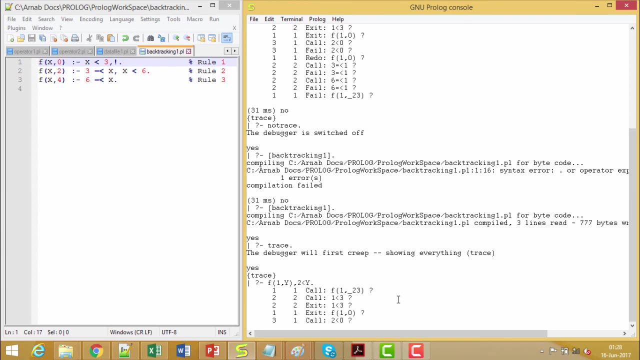 go. loneliness is the goal, so it is coming out with f 1: 0. so y has become 0 here. so after that we are having one cut, so that will get executed here. the next part of my query is 2 less than y. so 2 less than 0 is. 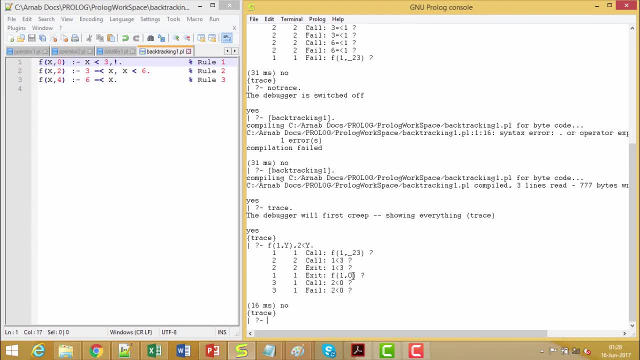 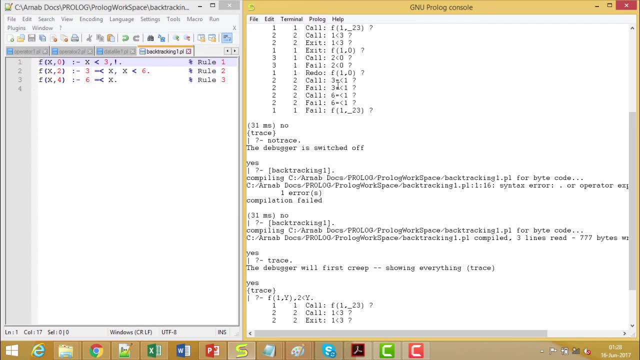 not true, so it is failing. and here you see the rest part which was tested earlier in this execution which was tested, that is, we're having this f 1, 0, we're having this one, so all the testing, whatever we had here, so that is not getting executed due to the presence of this cut.